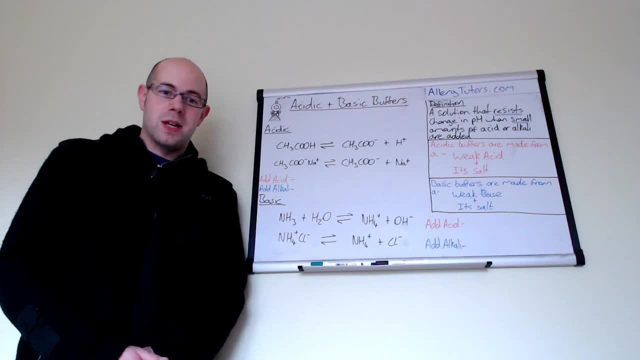 video. you should have a little bit more of a clearer idea of how these things work and why they're actually really useful, because they're used in such a large area. Even in your own blood there's buffer solutions, So we're just going to have a look at the 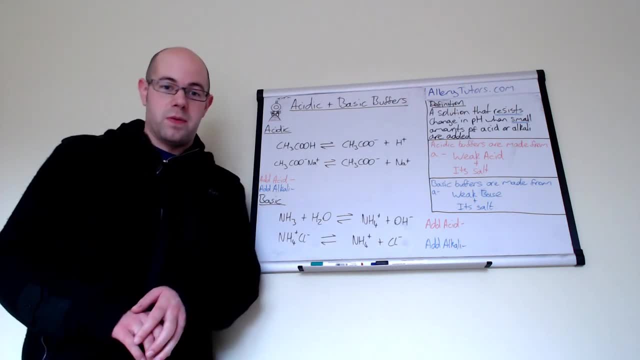 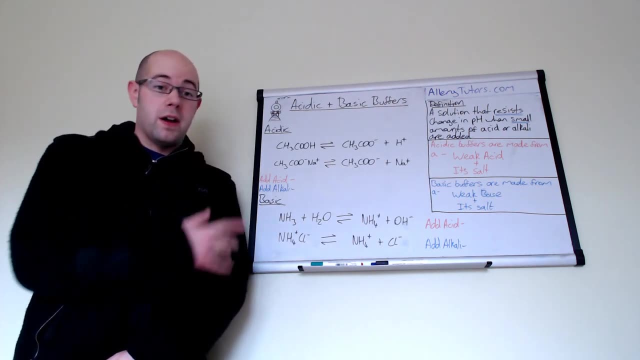 definition. first, I'm going to show you what an acidic buffer is and a basic buffer and basically show you how they work in terms of the chemical equations that I've got on the board. So a buffer- the definition of a buffer- is basically a solution that resists. 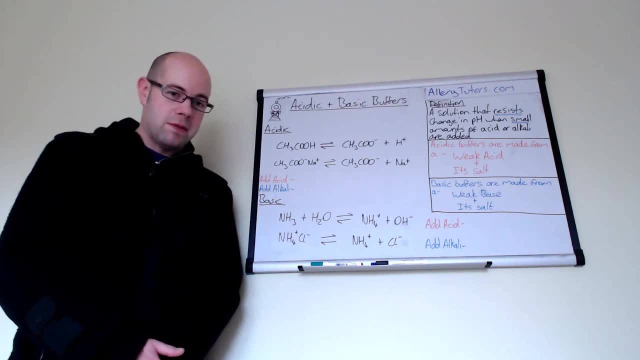 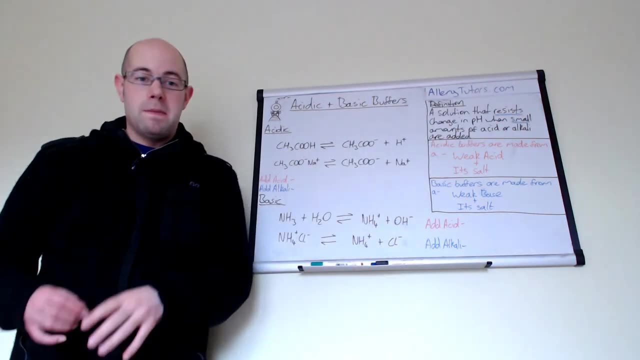 a change in pH when small amounts of acid or alkali are added to it. So the key words here are resists and small. It doesn't actually Okay. A buffer doesn't actually stop the pH from changing. It actually just slows it down. 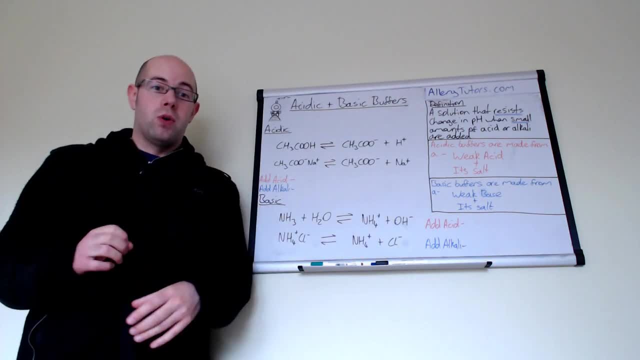 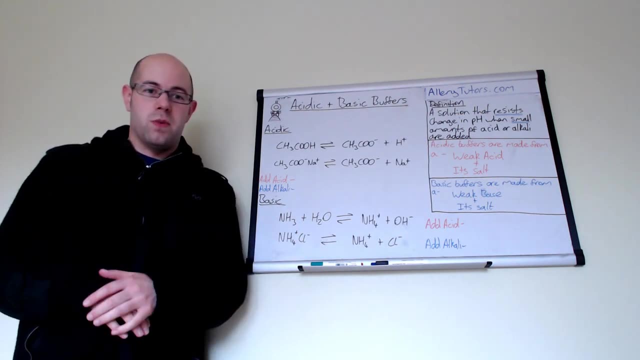 It resists it And it only does that if a small amount of acid or alkali is added. Buffers can't cope when you throw large amounts of acid or alkali in there and it just doesn't work. So it is restricted to certain criteria, but you do have to know the definition It's. 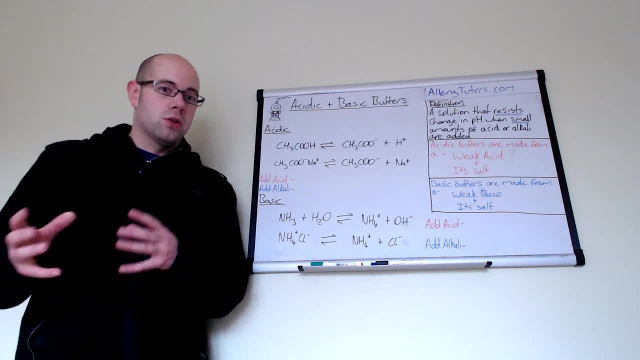 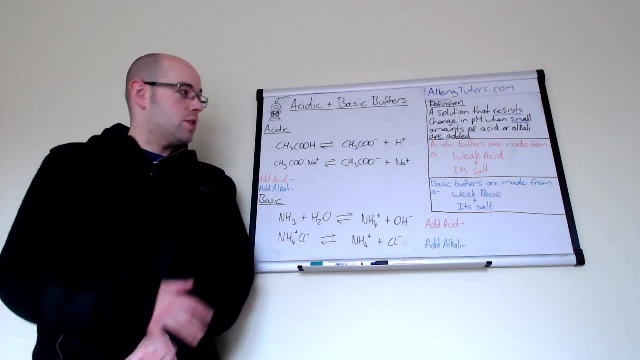 so so important. and actually understanding the definition also helps you to work out chemically what's happening to a buffer. So there's two ways in which you can make a buffer. So the first one is an acidic buffer, and these obviously keep a pH within the acidic range. 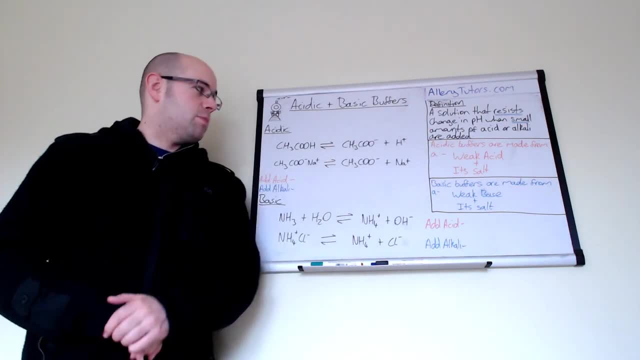 That's what acidic buffers do. So to make an acidic buffer you need a weak acid. So ethanoic acid, methanoic acid, anything like that, carboxylic acid and its salt. Normally it's like a sodium version of the acid, So sodium methanoate, for example, would be the. 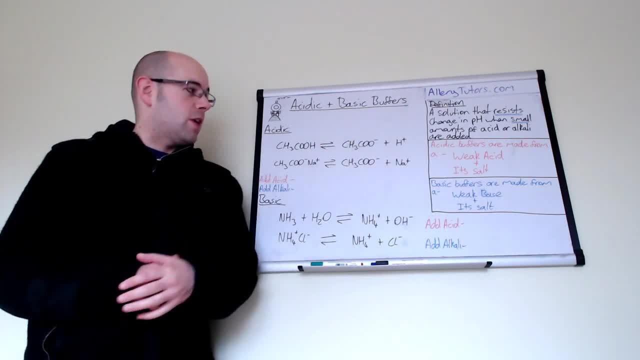 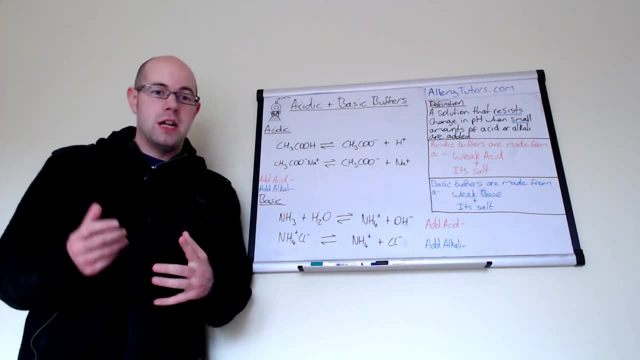 salt for ethanoic acid And a basic buffer is basically made from a weak base and its salt So a bit like the acid one, but using a weak base, And commonly it's ammonia. That's your weak base and the salt would be something like ammonium chloride. So these are the two. 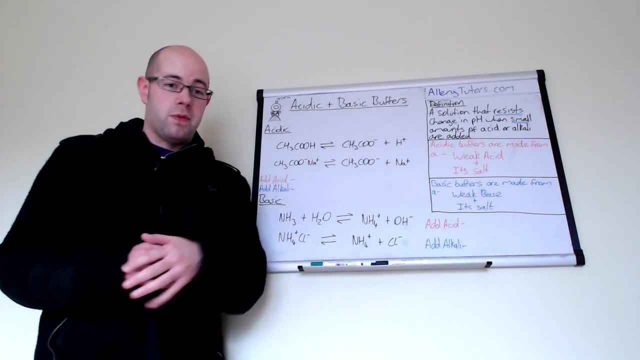 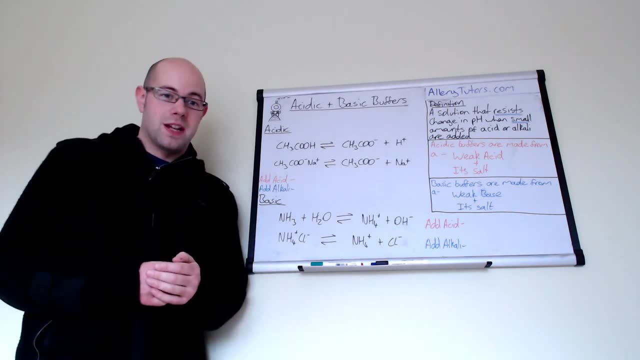 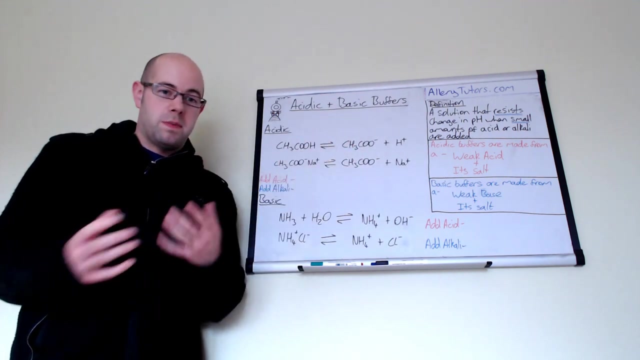 different types of buffers that you can have, And an acidic buffer basically tries to keep a substance at an acidic pH, So anything below 7.. And obviously a basic buffer keeps things in anything above pH 7.. So they have uses and it depends on what the use is. So for 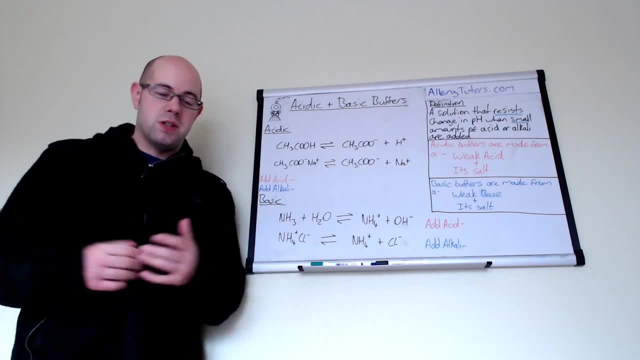 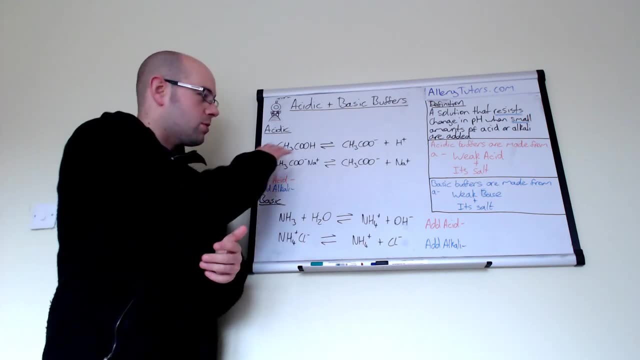 example, for shampoos, you would have a basic buffer, because shampoos need to be slightly alkaline. So we're going to have a look at this. first, I'm going to show you in two equations to show you what's happening. But these two equations are very strongly linked together. 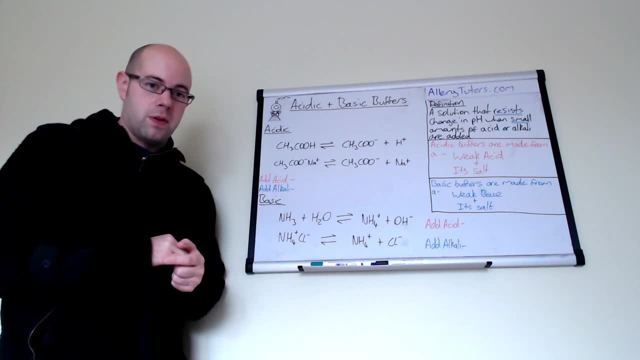 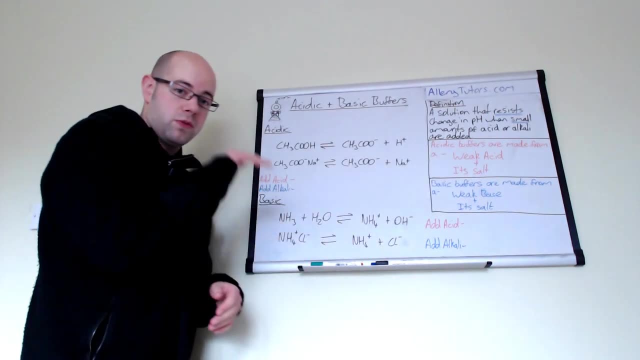 and you should see them as a pair rather than as individual equations. So here's our acidic buffer. Remember the definition? we said it's a weak acid and its salt. So we've got two equations showing that. So we've got the weak acid equation which is up here. So this is. 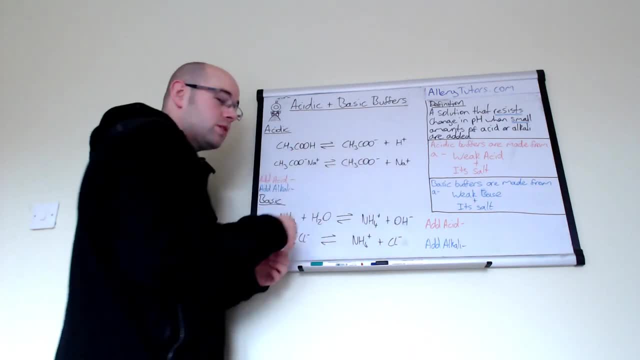 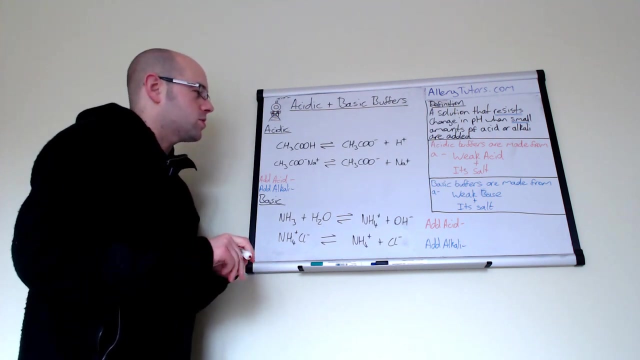 ethanoic acid. So ethanoic acid will dissociate to form ethanoate ions and H plus ions, And if we have to write down the relative concentrations of it, we can say that actually, because this is a weak acid, it dissociates very poorly, So it doesn't break up into its ions very. 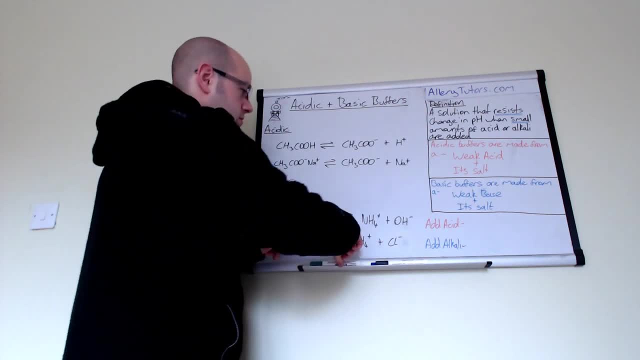 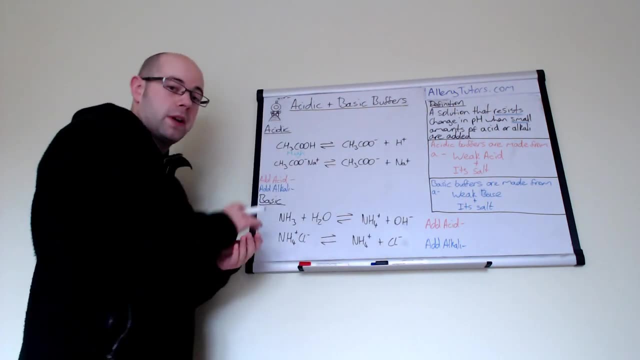 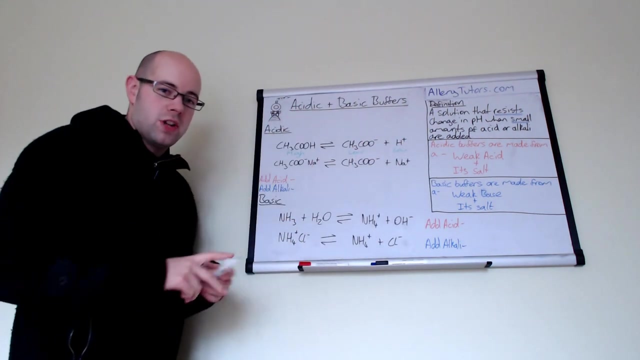 readily. So we can say in terms of the concentrations- and we'll do this in green so you can see the difference- So we have a high concentration of ethanoic acid and we have low concentrations of ethanoate and a low concentration of H plus, And that's because it doesn't dissociate. 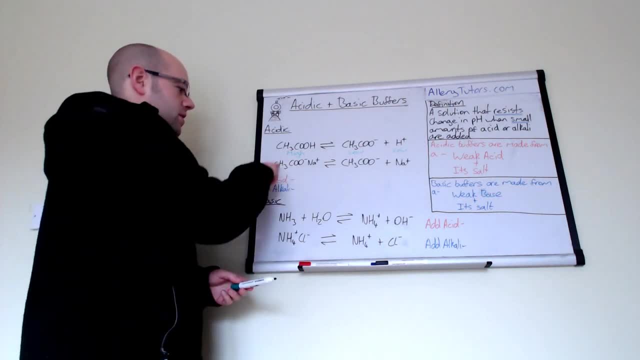 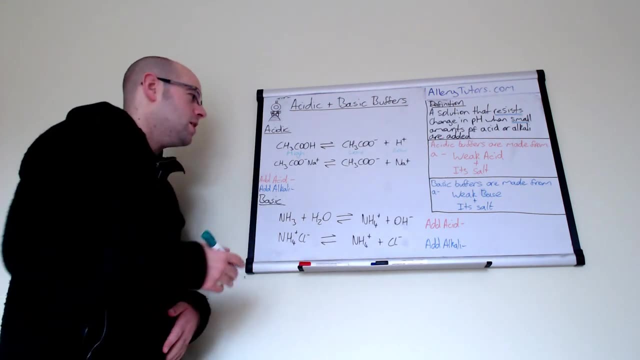 fully. If we look at the salt, though- and let's say we take the salt of ethanoic acid, So in this case I've picked sodium ethanoate. It could be potassium ethanoate, it could be lithium ethanoate, it doesn't really matter, But sodium ethanoate is the most common form that you. 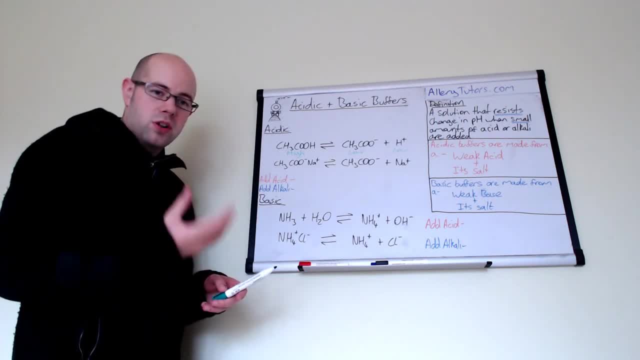 could use Now this salt when we dissolve it in water. obviously, all these things are in solution. That's what the buffers are. they're in solution And this breaks down the ethanoate. So we've got a lot of ethanoate, We've got a lot of ethanoate. We've got a lot of ethanoate. 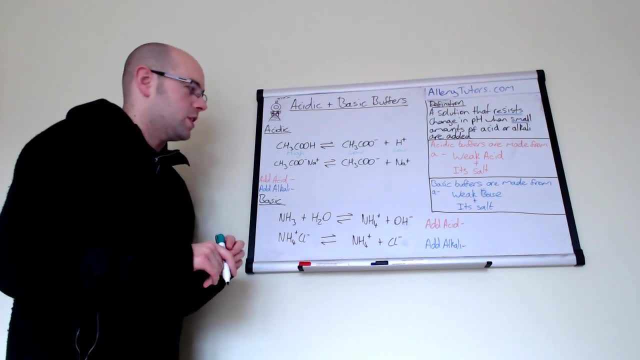 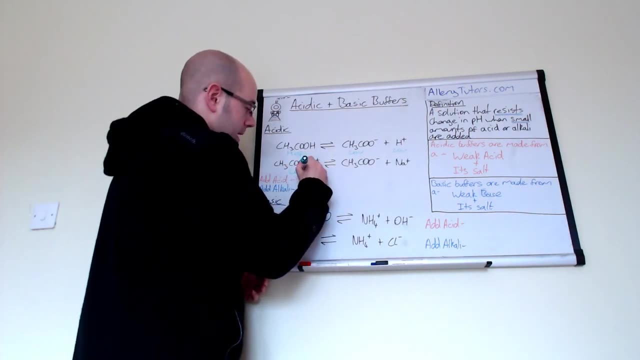 This breaks up readily. Most salts dissolve very readily within water, and so, therefore, this will break up into its ions very readily. So, in terms of this, we have low amounts of salt and we have high amounts of this, which is your ethanoate ion, which is similar, which 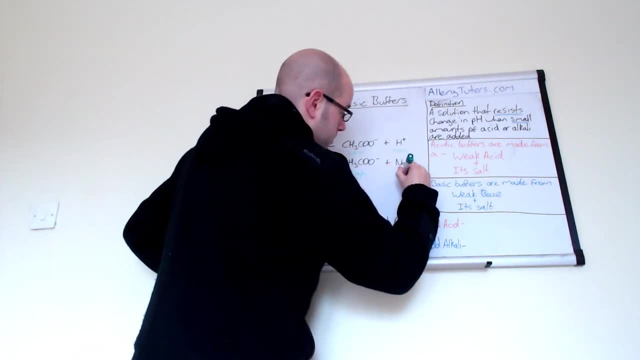 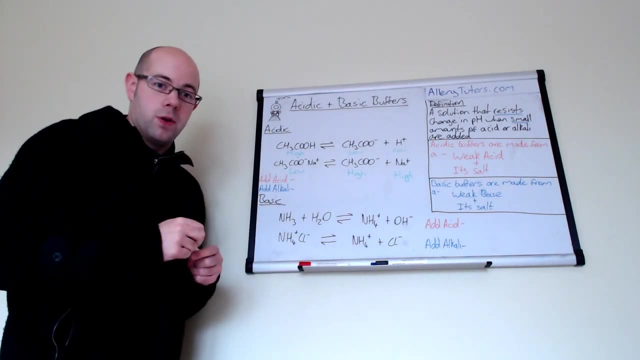 is the same as what we've produced in our acid, And we have high amounts of sodium ions as well. Now these two are mixed together, and when we mix them together, we actually form a buffer solution And these two are actually being thrown into a beaker and they actually exist together. 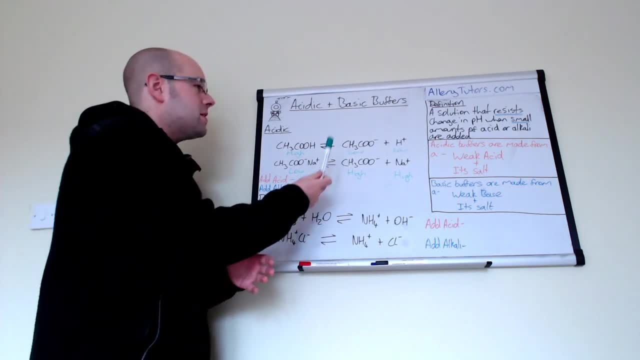 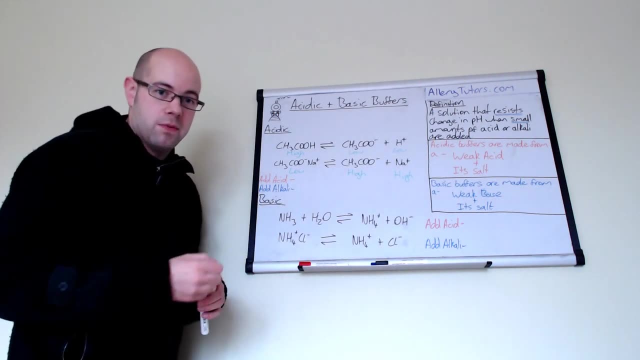 even though we've written them out as two separate equations. So, basically, a buffer is something that resists a change in pH when small amounts of acid or alkyl are added. So that's what we're going to find out. We're going to find out what happens when we add a small amount of acid and a small amount of alkyl. 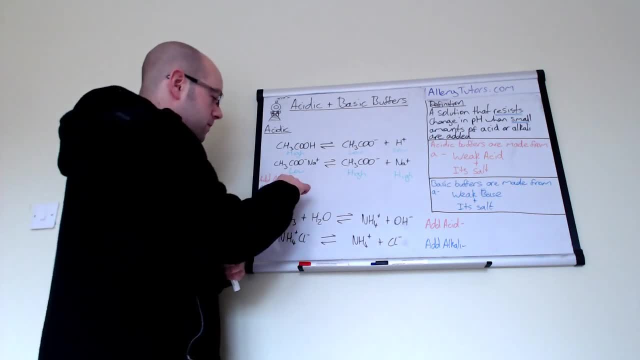 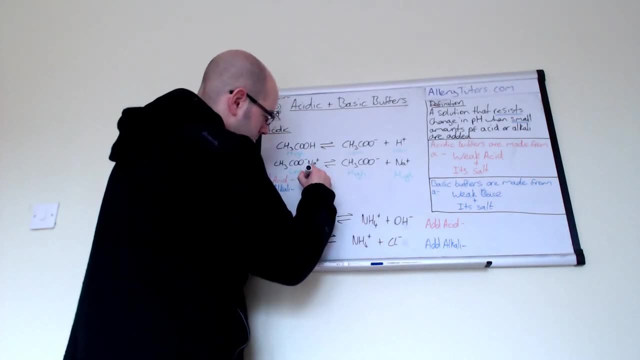 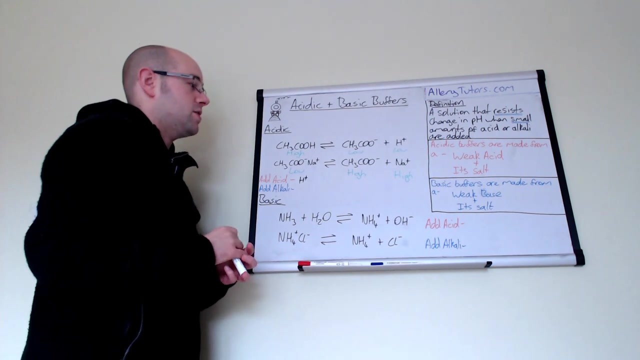 And we're going to explain this in terms of equilibrium. So if we add an acid, so an acid is obviously H+. So we're going to write this in this column: So acids are H+. So if we add an acid to this here, the H-plus ion is actually going to react with your ethanoate ions, which are over here. 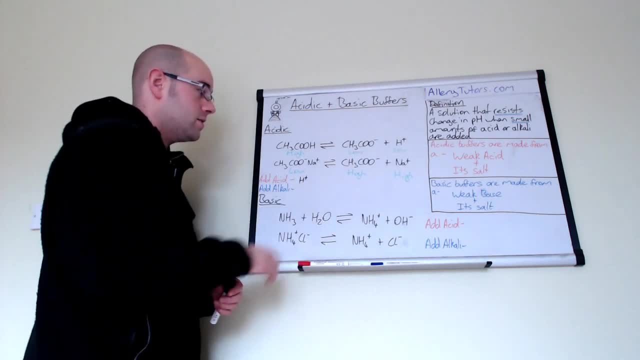 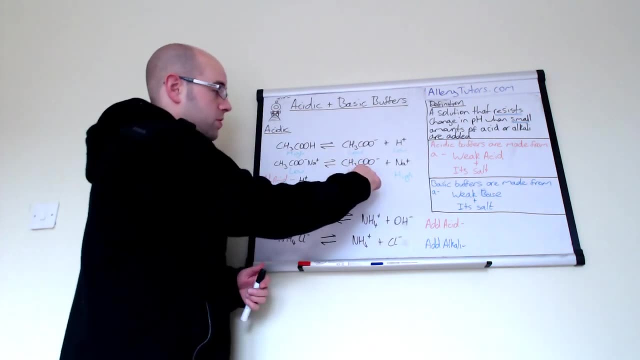 Now you can see that we have a large amount of ethanoate ions, which is here, And we have a small amount here, but that doesn't matter, because they're all in the same beaker, remember. So the H-plus will actually react with your ethanoate ions and it will produce this, which is ethanoic acid. 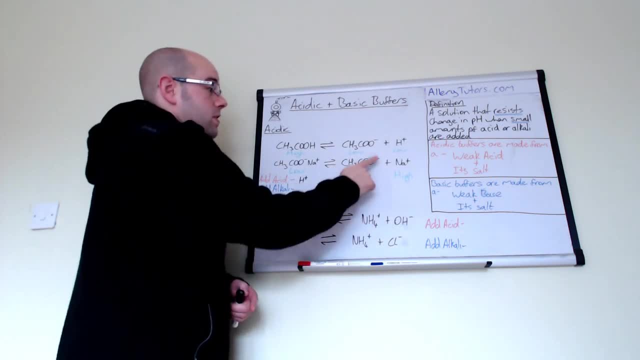 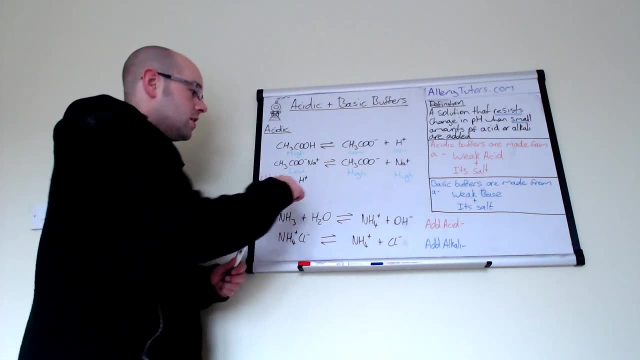 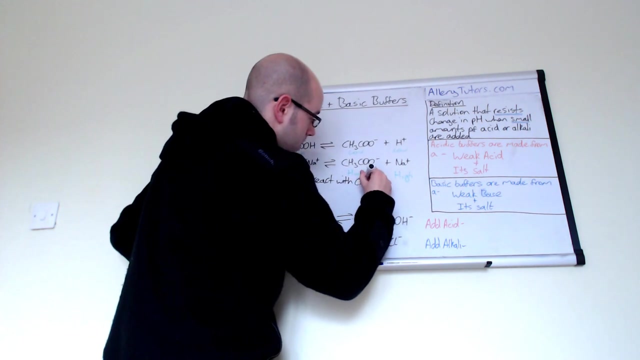 So by adding an acid, So by adding an acid, this actually effectively reacts with this to produce that. So we're absorbing or using up the H-plus ions that we've just added in. So the H-plus ions, they will react with a CH3, COO-. 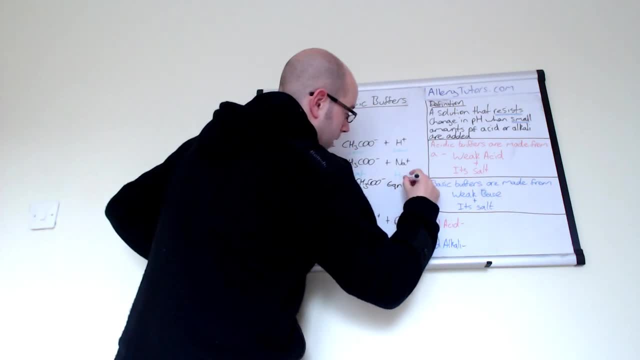 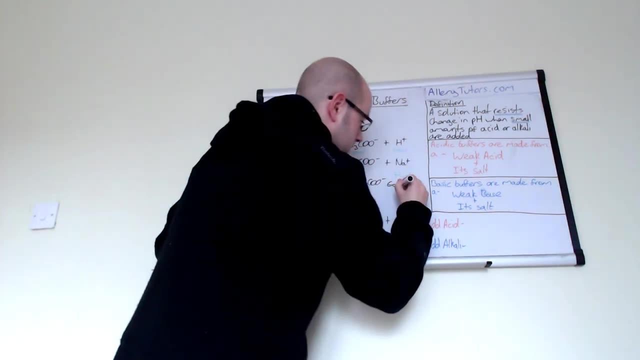 And then equilibrium will actually shift to the left. So I'm going to put now, we'll put in left, So equilibrium will shift to the left. So we're absorbing or using up the H-plus ions to produce more ethanoic acid ions. 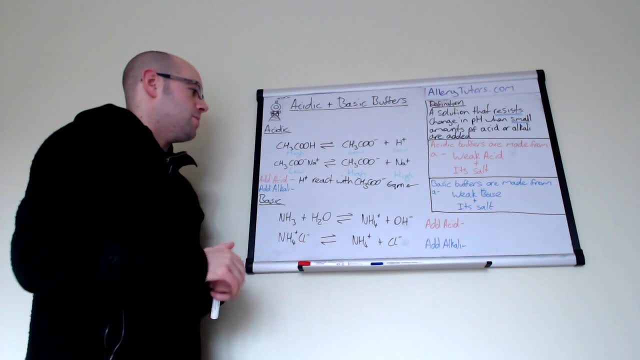 So because we have a high concentration of that, then this will effectively allow H-plus ions to be reacted, So that's a good thing. That's why the salt is there. So when you add an acid, you have a large amount of ethanoate ions to produce ethanoic acid. 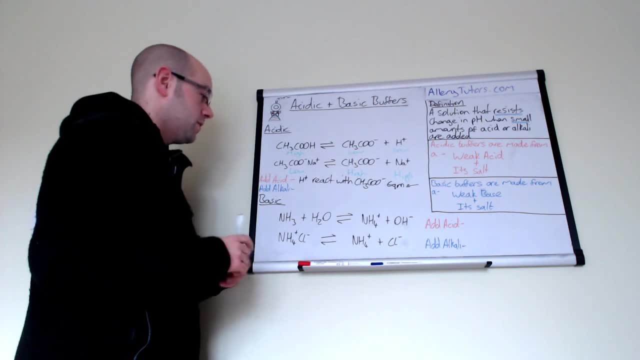 Now if we add an alkali, alkalis are obviously hydroxide ions, so OH-minus ions- Now OH-minus ions- will react. They will react with positive molecules or positive parts. So you can see we've got a large amount of sodium there. 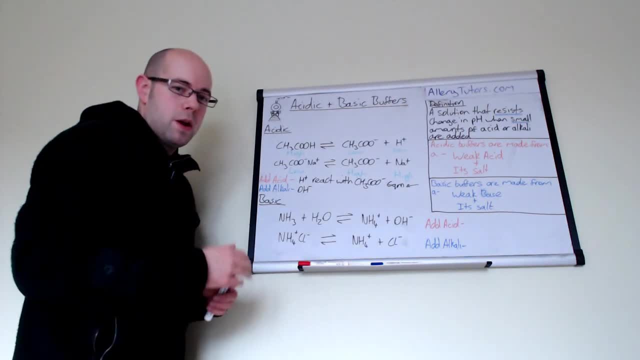 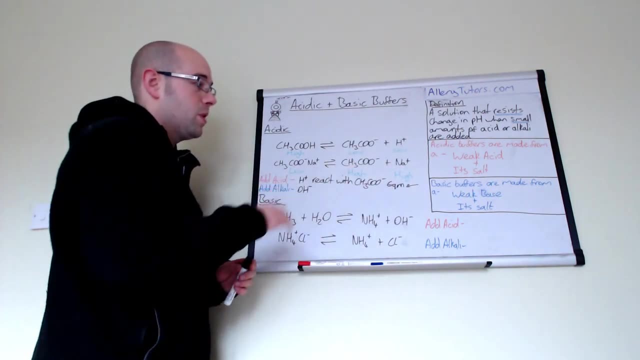 But if the hydroxide ion reacted with sodium, it would just break up and form sodium hydroxide again. Again, this is really soluble. So the hydroxide ion does react with sodium, but it actually doesn't play any role in terms of the buffer action. 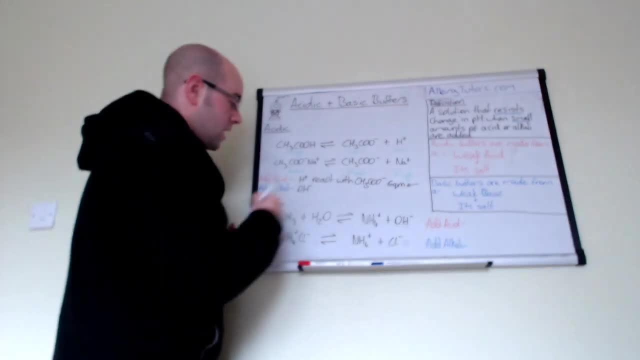 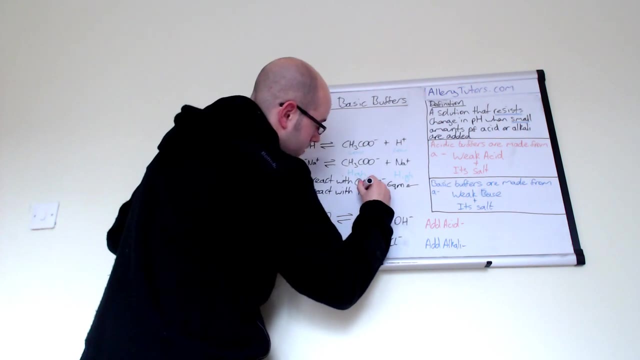 So what does play a role is the H-plus ion. So this, the hydroxide, actually reacts with, with the H-plus ion over here And you can see we've got a bit of a problem because we don't have a large amount of H-plus ions. 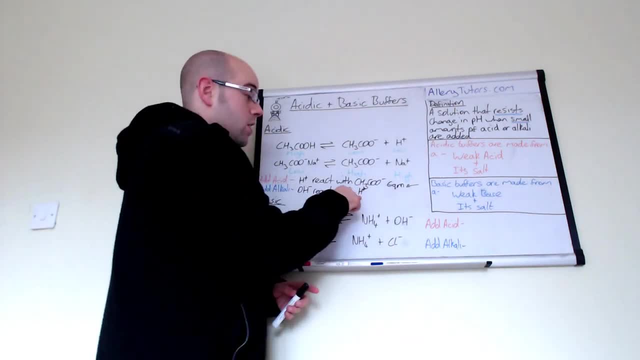 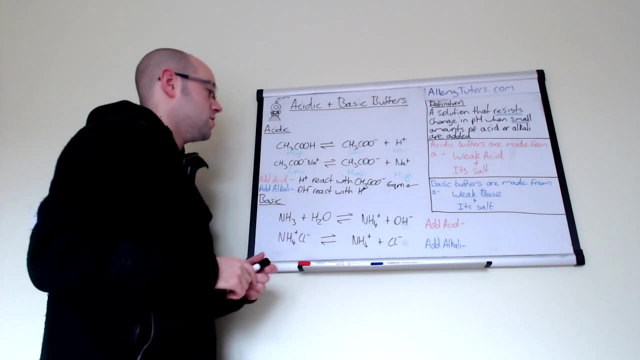 So the amount of hydroxide would very easily overwhelm the amount of H-plus ions that we've got here. But luckily we have a high amount of this, which is ethanoic acid, And so what happens is when the OH-minus reacts with your H-plus ions. 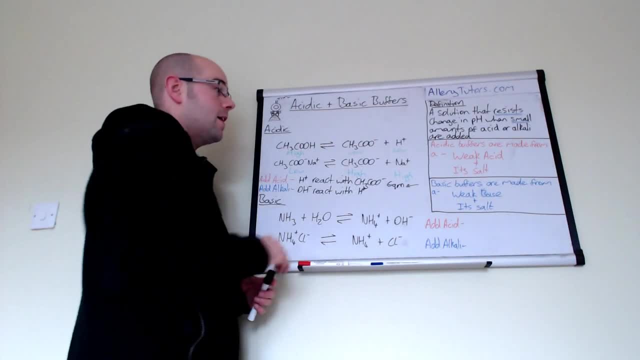 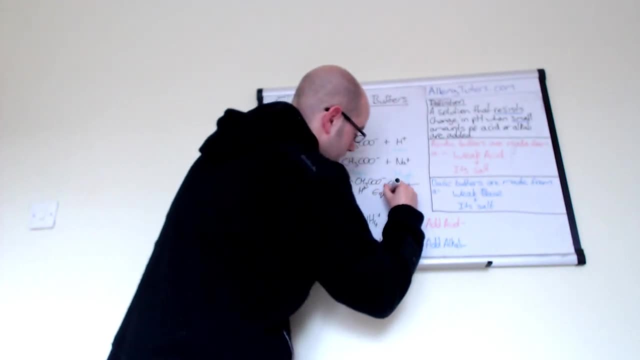 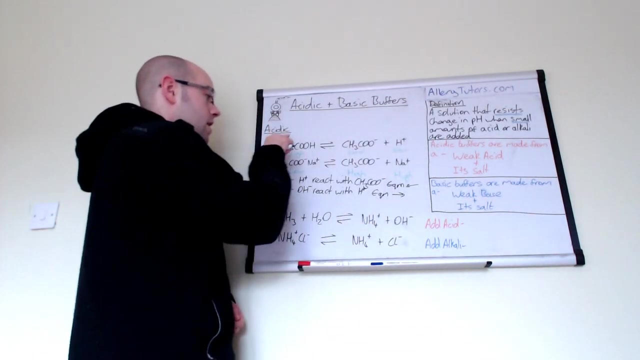 the ethanoic acid dissociates, to replace them H-plus ions back again. So OH-minus reacts with H-plus and the equilibrium will actually shift to the right, Because the OH-minus will react with your H-pluses, which are over here. 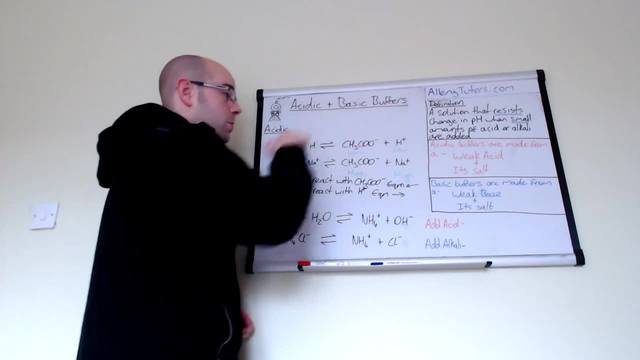 and this will break up or dissociate to form them back again. So according to the Chatelier's principle, if we remove or if we alter the amount of H-plus ions on there, the equilibrium will shift to try and oppose that change. So in other words, it'll shift to the right to put them back again. 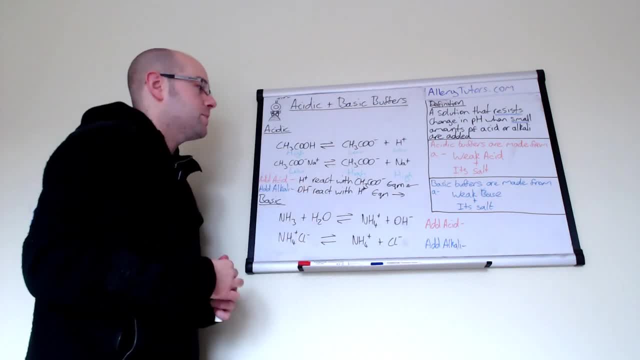 So that's what happens when we add hydroxide on there. So that's basically how that works for an acidic buffer, And it's really, really similar for a basic buffer as well. And so for a basic buffer, we've got ammonia and we've got water. 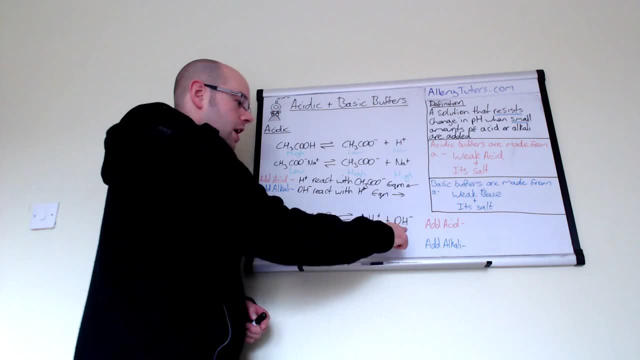 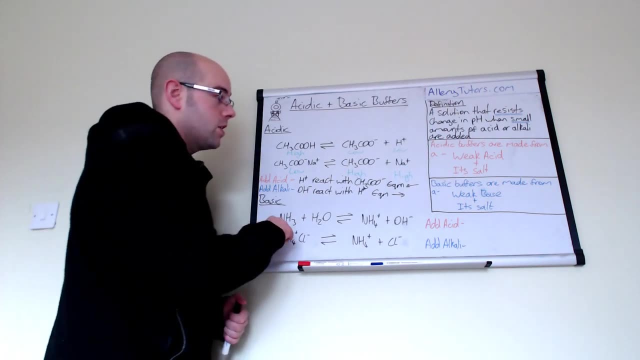 And these two will react together to form ammonium ion and hydroxide ion. Now, this is your, Obviously, this is your weak base, which reacts into form that, And we need its salt, And so its salt would be ammonium chloride. 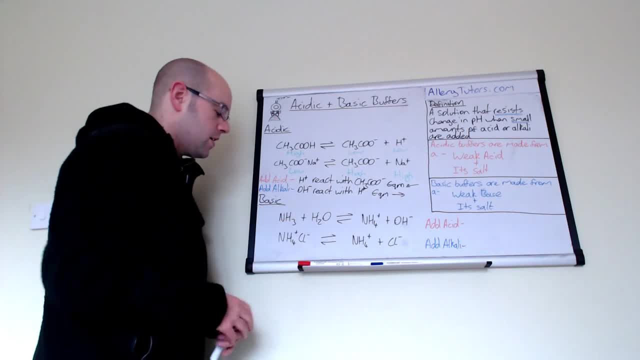 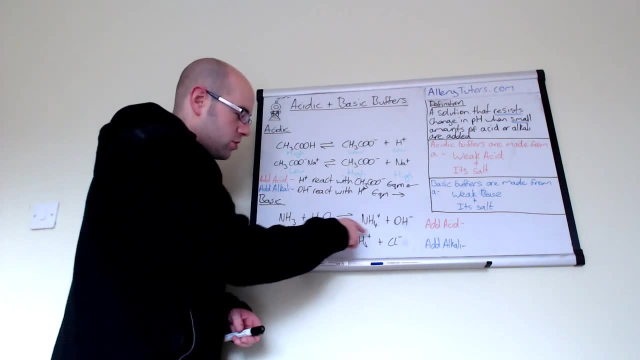 Again, it could be ammonium bromide, It could be ammonium iodide, It could be anything, But this is the most common salt that you could make from ammonia. So ammonium chloride, And again this dissociates fully to form ammonium and chloride ions. 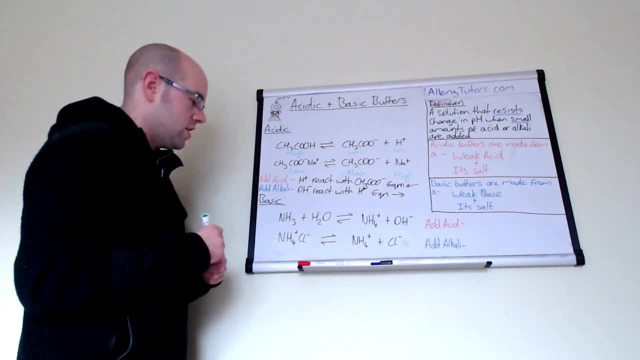 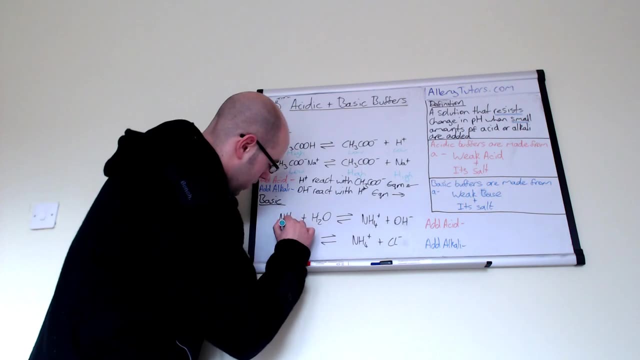 So, just like what we've done up here, we're going to write down our concentrations. So we have: This is a weak base, so it doesn't dissociate very well, So we actually have a high amount of these two. The water is just there as well. 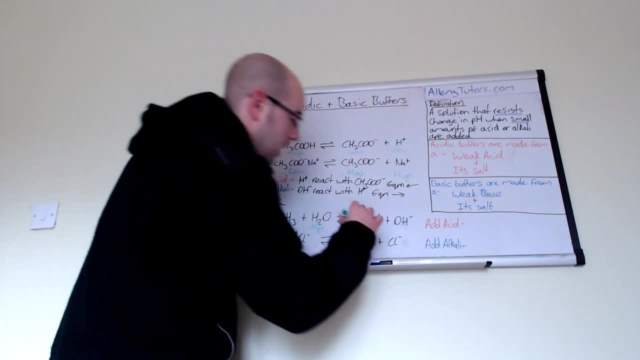 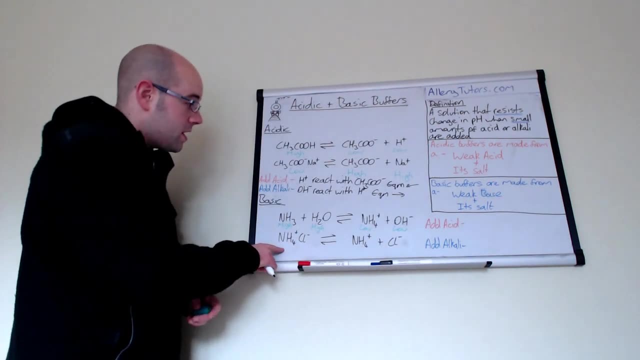 I'll put high on there as well. You'll have a large amount of that And you'll actually have low amounts of ammonia, of ammonium and low amounts of hydroxide. On this side, ammonium chloride is the salt. 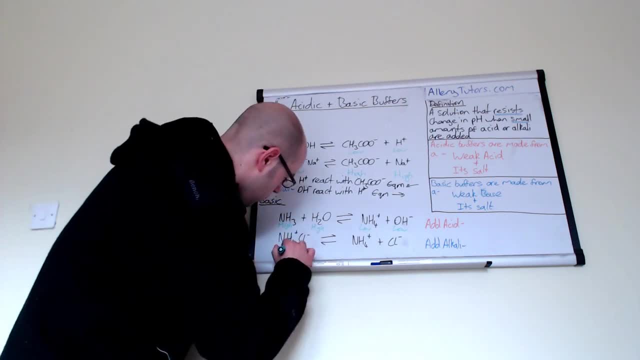 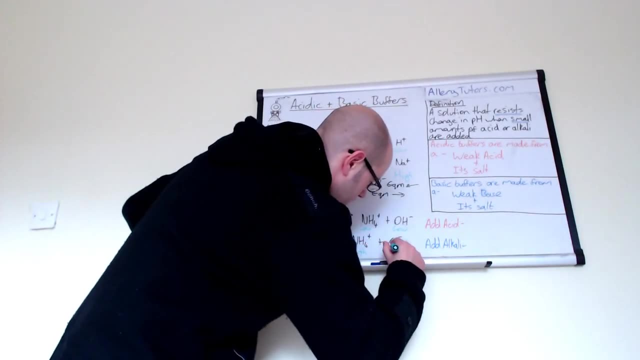 Salts dissociate readily when they're in solution, So you won't have a large concentration of that. So we're going to put low there. And because it dissociates quite readily, obviously we're going to produce high amounts of the ions that it breaks up into because it dissociates freely. 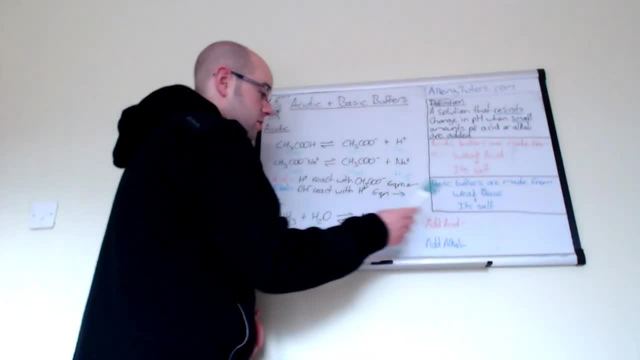 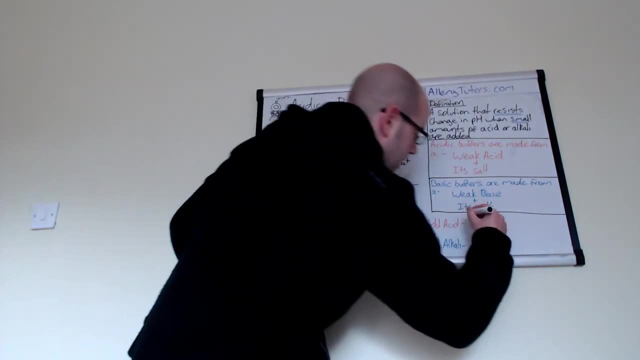 Now if we do a test on these, So if we add an acid and alkali, we need to work out what's actually going on. So if we add an acid, Now again, acid is H plus. These two are mixed together in the same beaker. 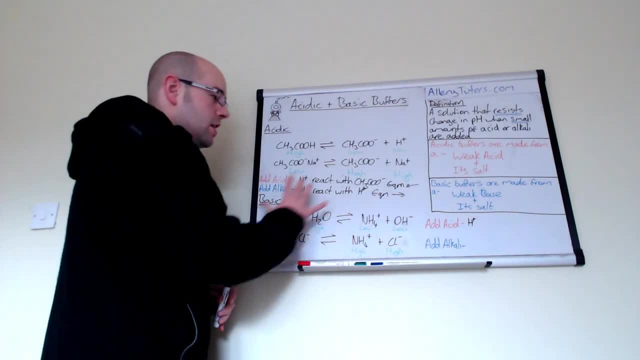 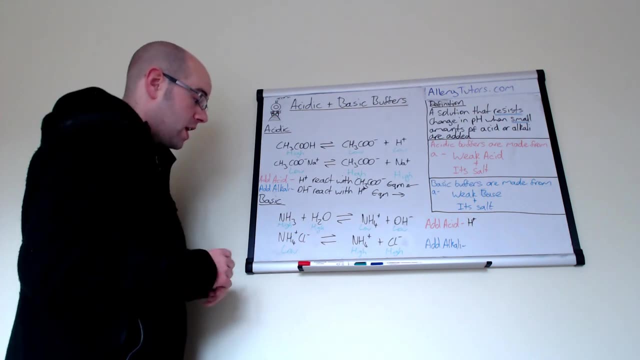 So if you imagine these two are completely mixed and we have all these ions floating around in the same beaker, If we add an acid which is H plus, the acid will actually react with something that's negatively charged And in this case it will react with the. 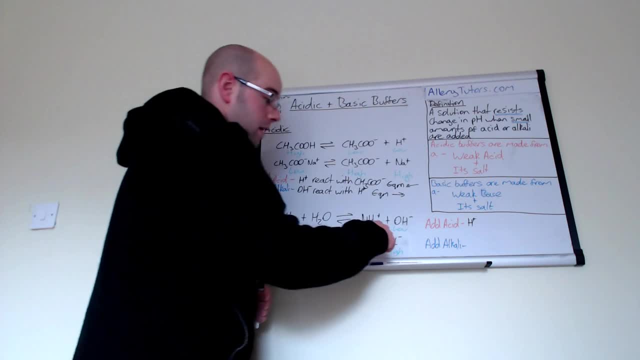 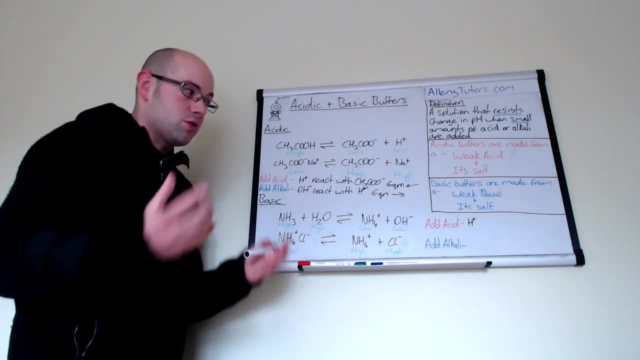 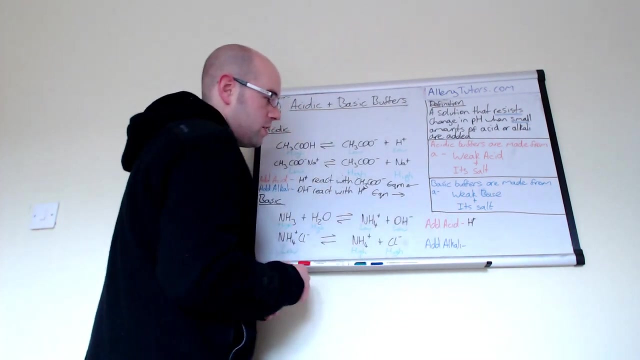 The, The OH minus. Again, if it reacted with the Cl minus it would produce HCl, which again dissociates as being an acid that will dissociate freely and just reform H plus and Cl minus back again. So instead what happens is the H plus reacts with the OH minus. 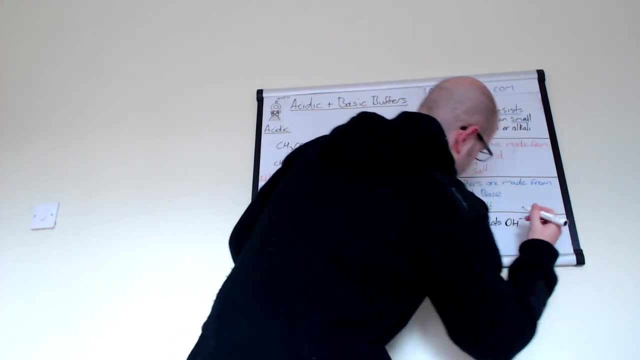 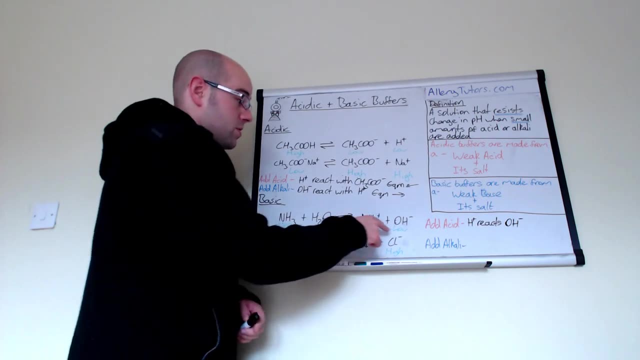 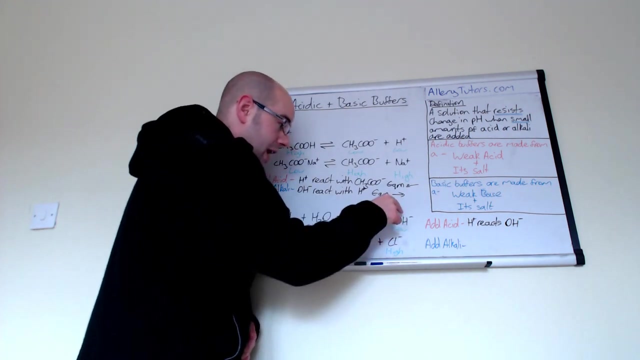 So we've got that there- Reacts with the OH minus, And when it does that, obviously we don't have a high concentration of this. So what actually happens is it reacts. It reacts with the OH minus, But this Because we have high amounts of these two here. these two will react to try and replace. 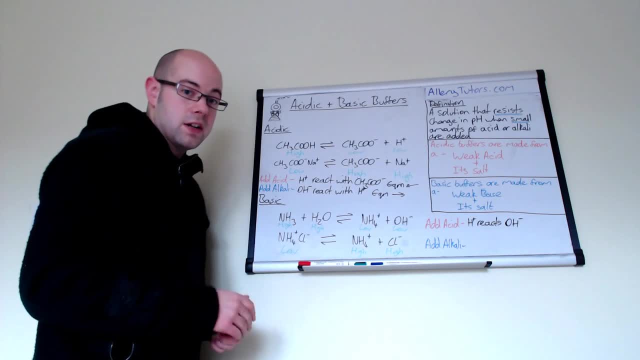 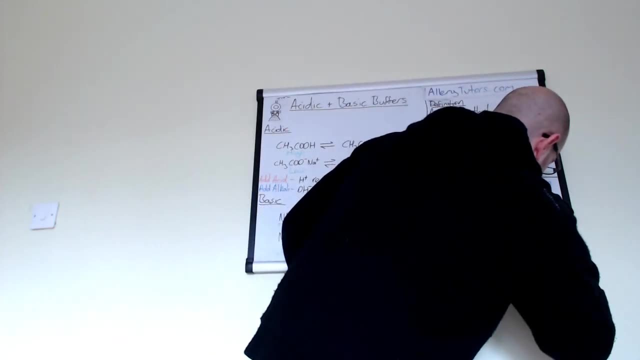 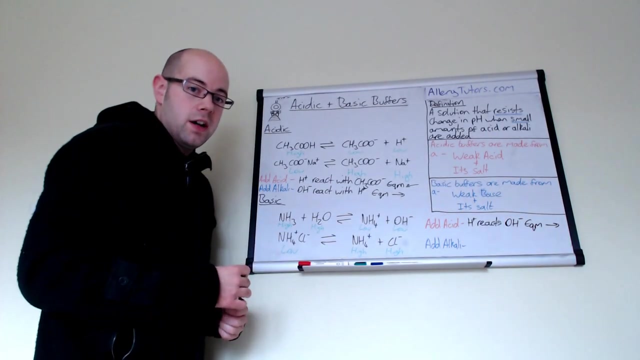 the OH minuses that the H plus has just reacted. So, again, according to Le Chatelier's principle, equilibrium will shift to the right, And so that is what we're going to put on there. Equilibrium shifts to the right to replace the hydroxide ions that your H plus has added.